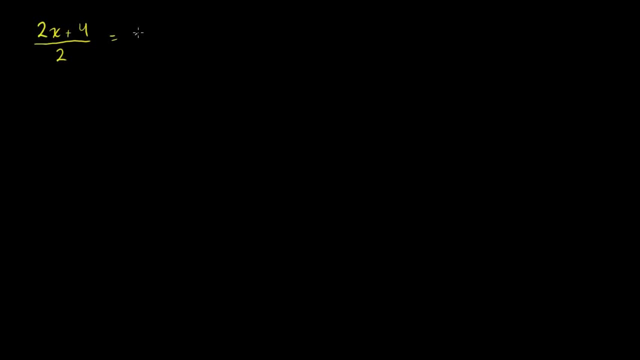 And this would be equal to what? This would be equal to x plus 2.. Let me write it this way: If you divide this by 2, it becomes an x. You divide the 4 by 2, it becomes a 2.. 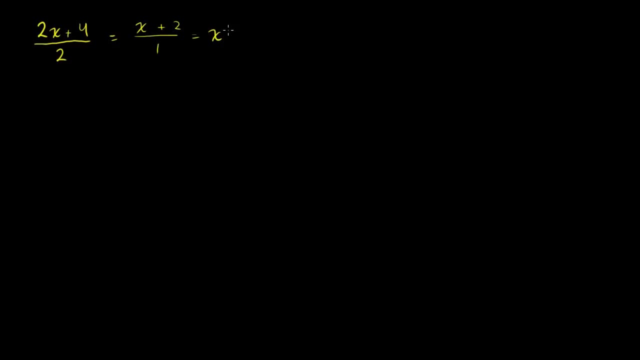 If you divide the 2 by 2,, you get a 1.. So this is equal to x plus 2, which is pretty straightforward. I think The other way is you could have factored a 2 out of here and 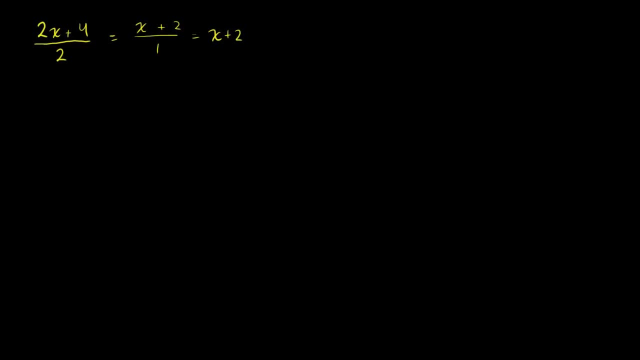 then those would have canceled out. But I'll also show you how to do it using algebraic long division, Which is a bit of overkill for this problem. but I just want to show you that it's not fundamentally anything new, It's just a different way of doing things. 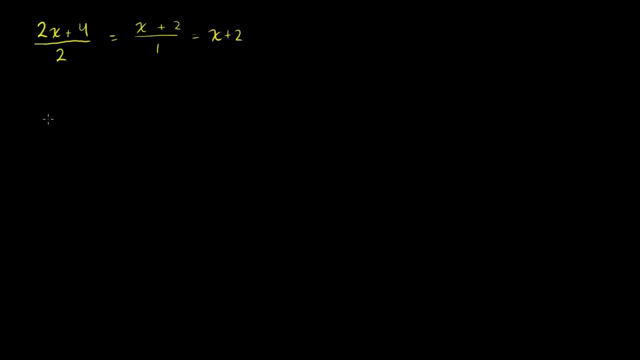 But it's useful for more complicated problems. So you could have also written this as 2 goes into 2x plus 4, how many times? And you would perform this the same way. you would do traditional long division. You'd say 2,, you'd always start with the highest degree. 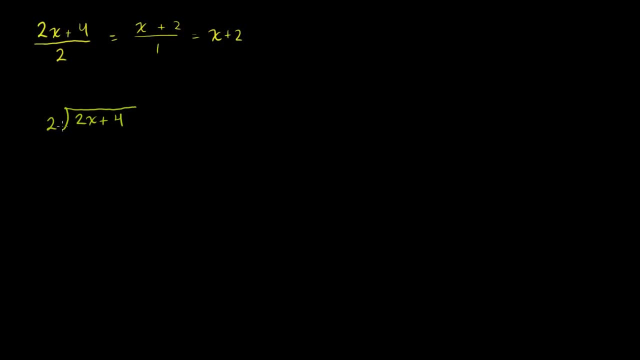 term 2 goes into the highest degree term. You would ignore the 4.. 2 goes into 2x. how many times? Well, it goes into 2x x times And you put the x in the x place. x times 2 is 2x. 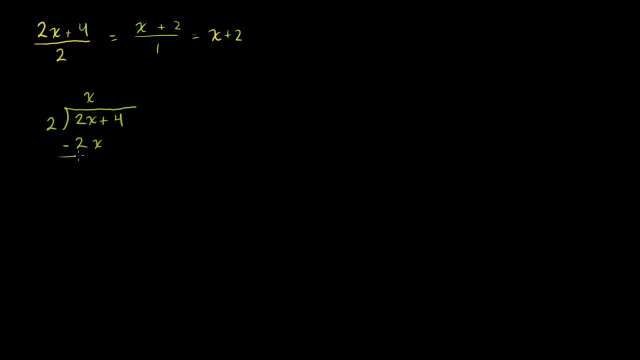 And just like traditional long division, you now subtract. So 2x plus 4 minus 2x is what It's 4, right. And then 2 goes into 4. how many times It goes into 2 times a positive 2 times? 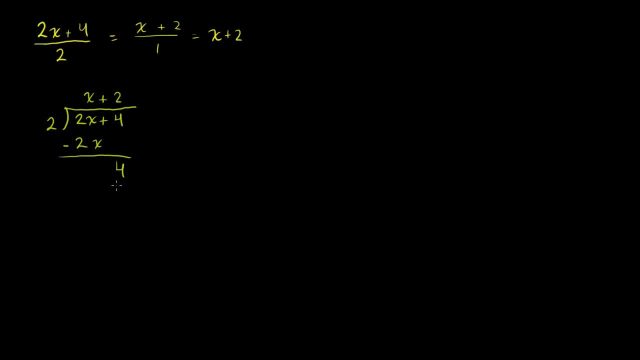 Put that in the constants place 2 times 2 is 4.. You subtract Remainder 0. So this might seem overkill for what was probably a problem that you already knew how to do, and do it in a few steps. 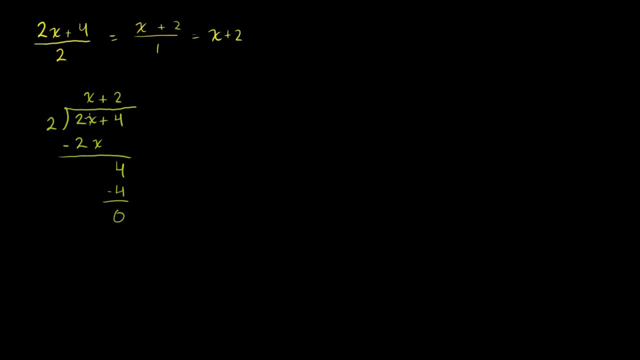 But we're now going to see that this is a very generalizable process. You can do this really for any degree polynomial, dividing into any other degree polynomial. Let me show you what I'm talking about. So let's say we wanted to divide x plus 1 into. 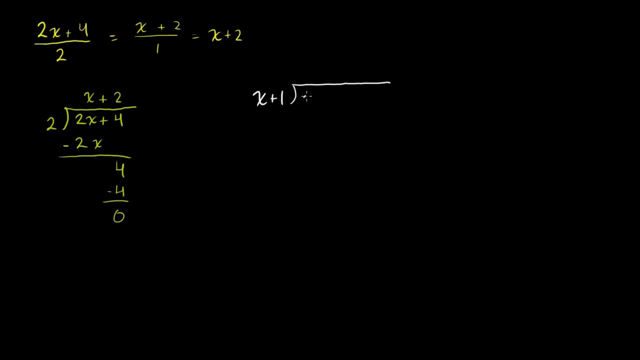 x plus 1 into x squared plus 3x plus 6.. So what do we do here? So you look at the highest degree term here, which is an x, And you look at the highest degree term here, which is an x squared. 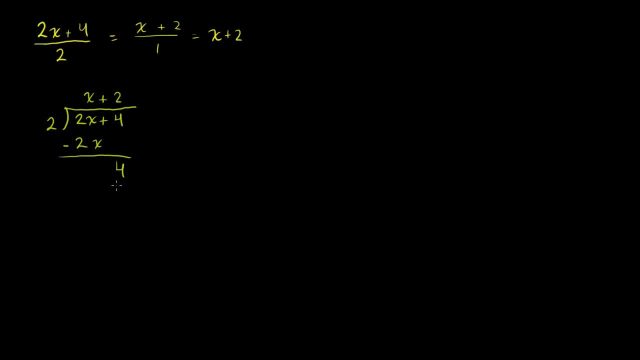 Put that in the constants place 2 times 2 is 4.. You subtract Remainder 0. So this might seem overkill for what was probably a problem that you already knew how to do, and do it in a few steps. 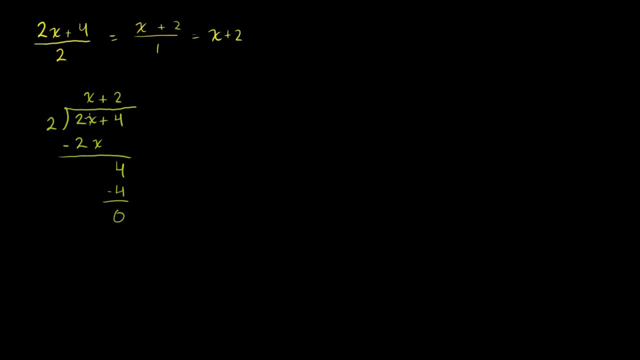 But we're now going to see that this is a very generalizable process. You can do this really for any degree polynomial, dividing into any other degree polynomial. Let me show you what I'm talking about. So let's say we wanted to divide x plus 1 into. 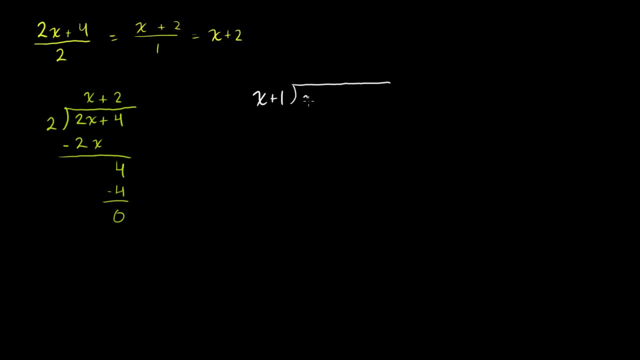 x plus 1 into x, squared plus 3x plus 3x plus 6.. So what do we do here? So you look at the highest degree term here, which is an x, And you look at the highest degree term here. 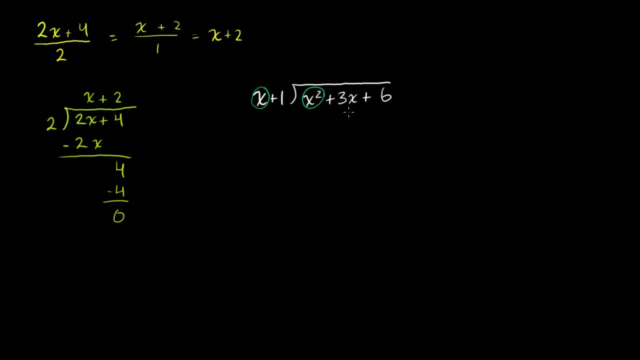 which is an x squared, So you can ignore everything else, And that really simplifies the process. And you say: x goes into x squared. how many times? Well, x squared divided by x is just x. right, Right, Right Right. 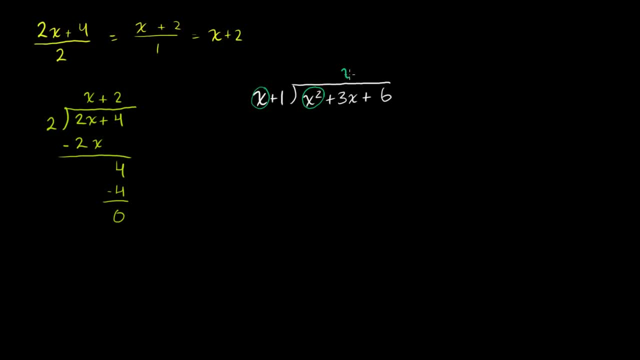 So x goes into x, squared x times, And you put it in the x place. This is the x place right here, Or the x to the first power place. So x times x plus 1 is what? x times x is x squared. 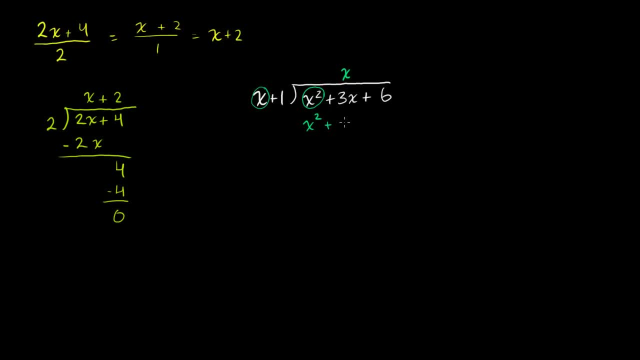 x times 1 is x, So it's x squared plus x. And just like we did over here, we now subtract, And what do we get? x squared plus 3x plus 6 minus x squared. Let me be very careful. 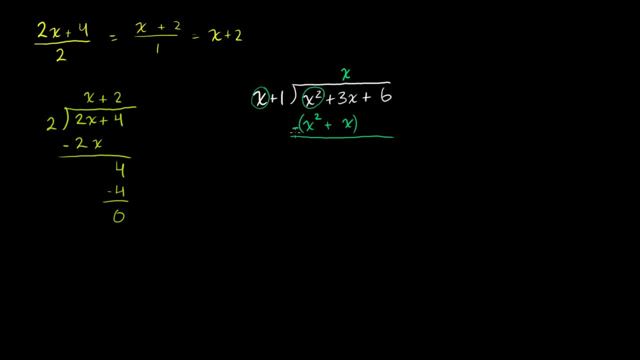 This is minus x squared. This is minus x squared plus x. Don't want to make sure that negative sign only applies to this whole thing. So x squared minus x squared those. cancel out. 3x is going to be a minus x. 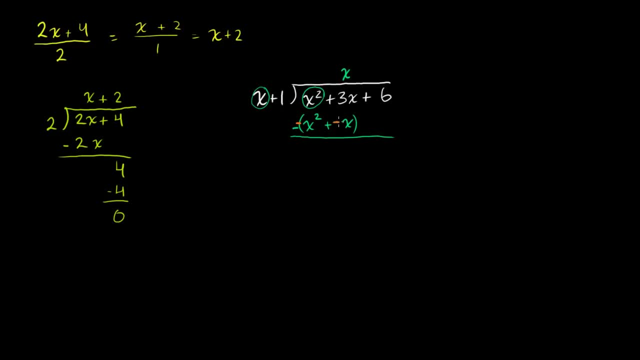 Let me put that sign there. So this is minus x, squared minus x. just to be clear, We're subtracting the whole thing: 3x minus x is 2x, And then you bring down the 6. Or 6 minus 0 is nothing. 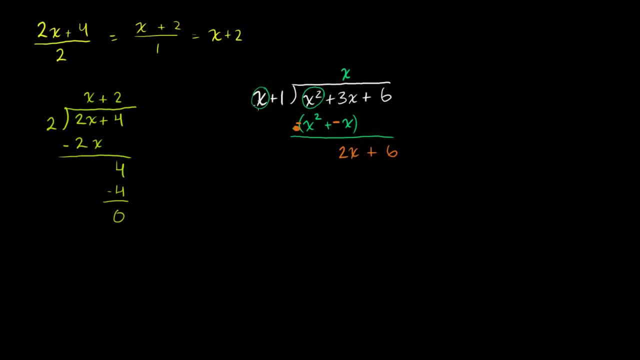 So 2x plus 6.. Now you look at the highest degree term, an x and a 2x. How many times does x go into 2x? It goes into it two times. 2 times x is 2x. 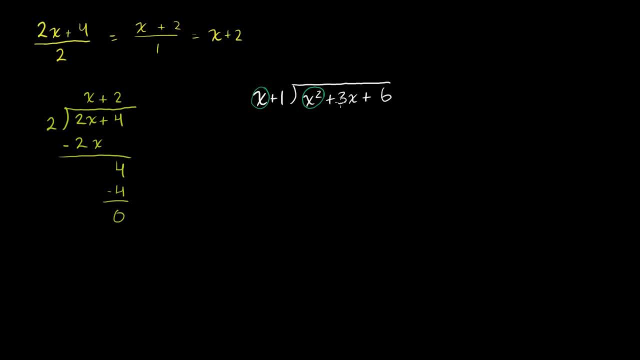 So you can ignore everything else, And that really simplifies the process. And you say: x goes into x squared. how many times? Well, x squared divided by x is just x, right, Right, Right, Right. So x goes into x squared x times. 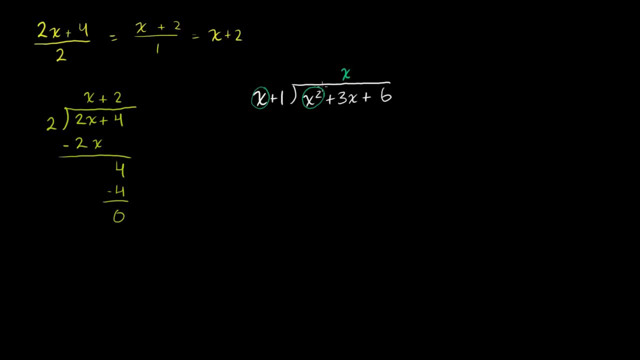 And you put it in the x place. This is the x place right here, Or the x to the first power place. So x times x plus 1 is what. x times x is x. squared x times 1 is x. So it's x squared plus x. 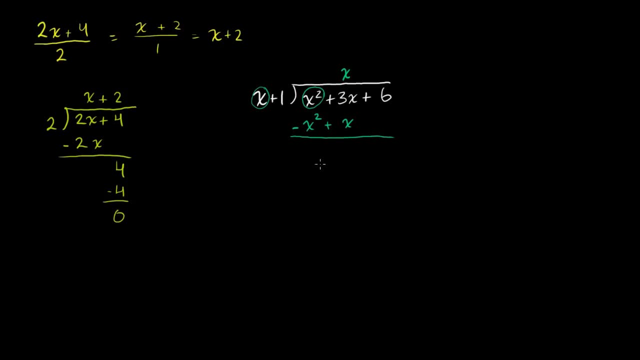 And, just like we did over here, we now subtract, And what do we get? x squared plus 3x plus 6 minus x squared. Let me be very careful: This is minus x squared. This is minus x squared plus x. 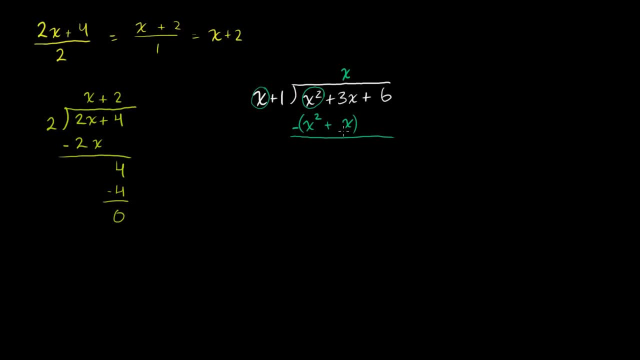 Don't want to make sure that negative sign only applies to this whole thing. So x squared minus x squared those cancel out 3x is going to be a minus x. Let me put that sign there. So this is minus x squared minus x, just to be clear. 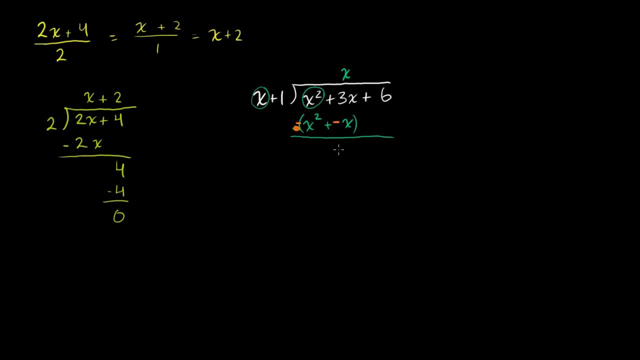 We're subtracting the whole thing: 3x minus x is 2x, And then you bring down the 6. Or 6 minus 0 is nothing, So 2x plus 6.. Now you look at the highest degree term: an x and a 2x. 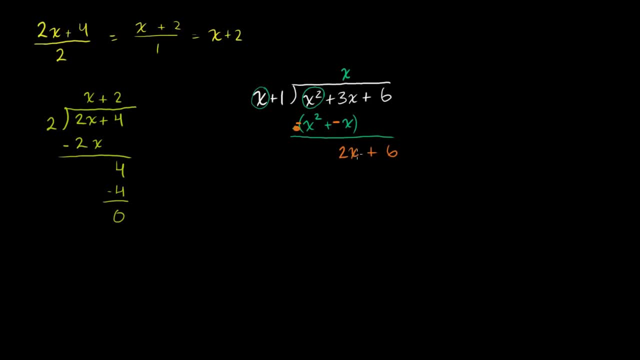 How many times does x go into 2x? It goes into it two times. 2 times x is 2x. 2 times 1 is 2.. So we get: 2 times x plus 1 is 2x plus 2.. 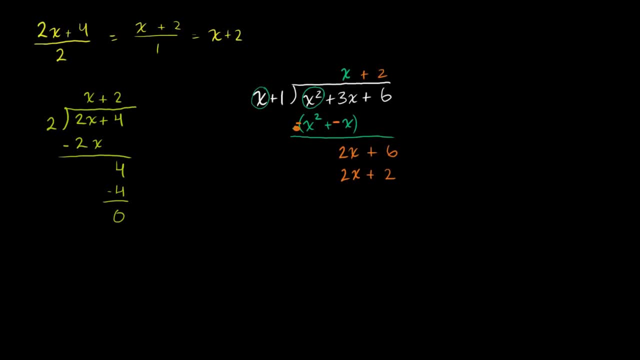 But we're going to want to subtract this from this up here, So we're going to subtract it. Instead of writing 2x plus 2, we could just write Negative 2x minus 2. And then add them. These guys cancel out. 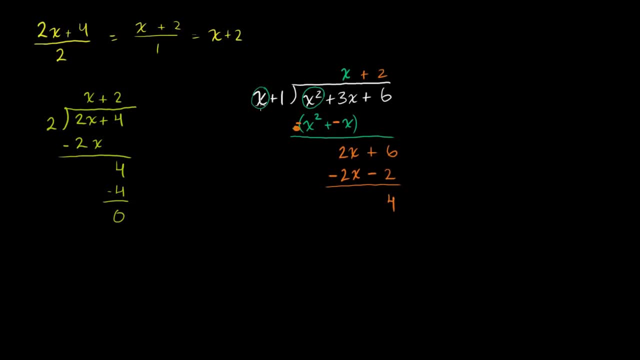 6 minus 2 is 4.. And how many times does x go into 4?? Well, we could just say that 0 times, Or we could say that 4 is the remainder. So if we wanted to rewrite x squared plus 3x plus 6 over, 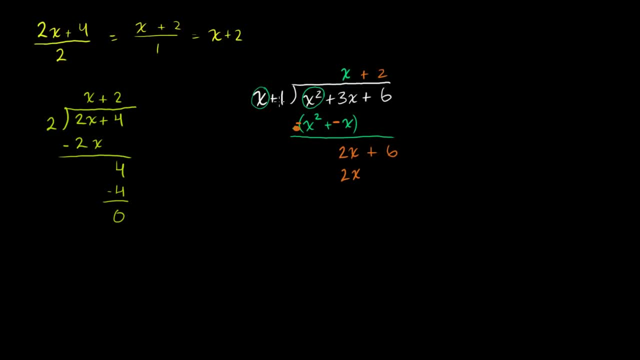 2 times 1 is 2.. So we get: 2 times x plus 1 is 2x plus 2.. But we're going to want to subtract this from this up here, So we're going to subtract it Instead of writing 2x plus 2, we could just. 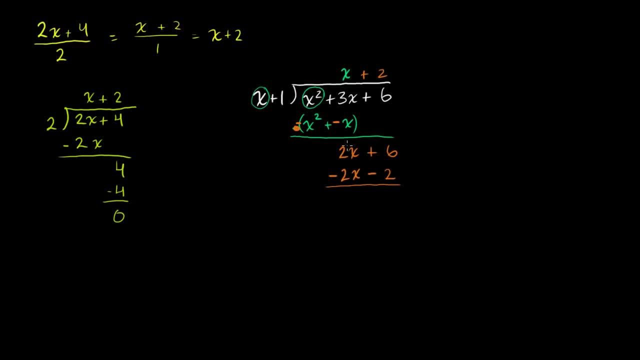 write negative 2x minus 2, and then add them. These guys cancel out: 6 minus 2 is 4.. And how many times does x go into 4?? Well, we could just say that 0 times, or we could say that: 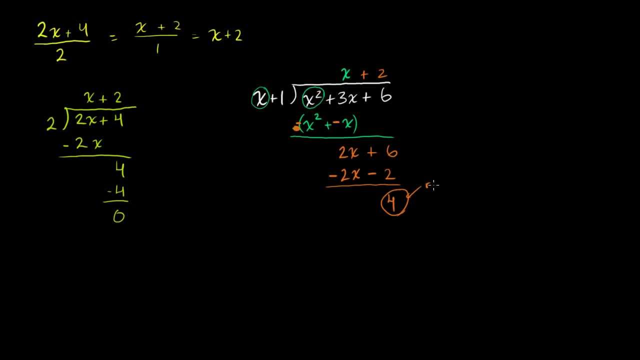 4 is the remainder. So if we were to rewrite, so if we wanted to rewrite x squared plus 3x plus 6 over x plus 1.. Notice, this is the same thing as x squared plus 3x plus 6 divided by x plus 1.. 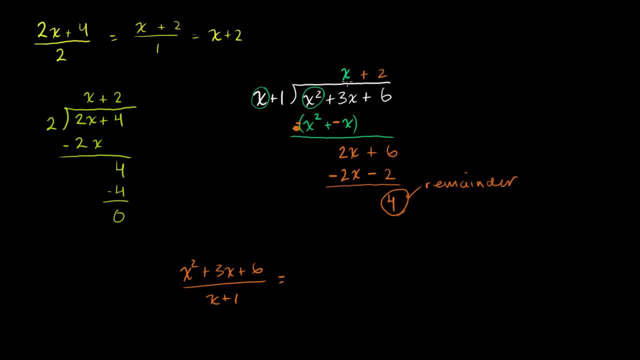 This thing. divided by this, We can now say that this is equal to x plus 2.. It is equal to x plus 2 plus the remainder divided by x plus 1, plus 4 over x plus 1.. This right here and this right here are equivalent. 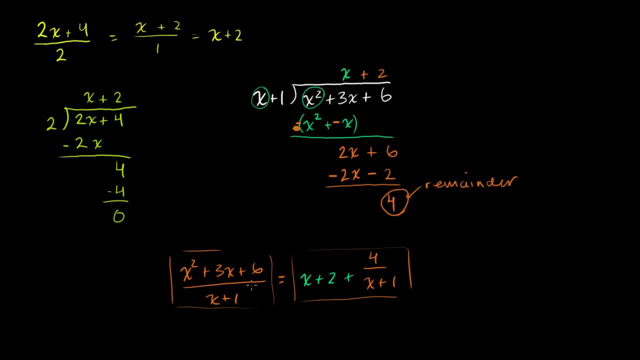 And if you wanted to check that, if you wanted to go from this back to that, what you could do is multiply this by. you could multiply it by x plus 1 over x plus 1, and then add the two. So this is the same thing as x plus 2.. 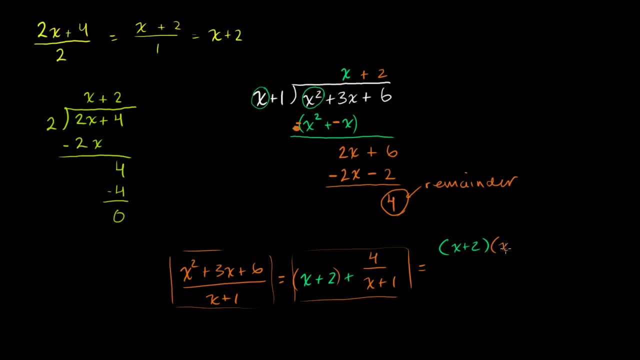 And I'm just going to multiply that times x plus 1 over x plus 1, right, That's just multiplying it by 1.. And then to that add 4 over x plus 1.. I did that, so I have the same common denominator. 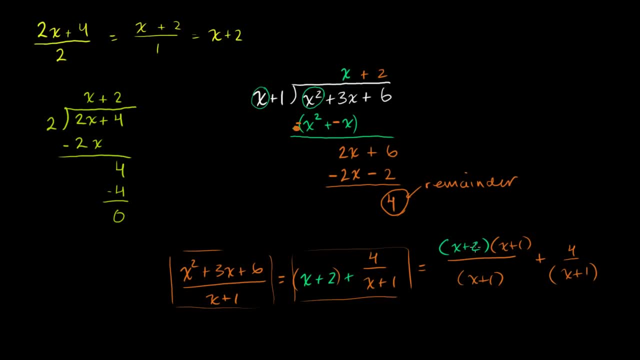 And when you perform this addition right here, when you multiply these two binomials and then add the 4 up here, you should get x squared plus 3x plus 6.. Let's do another one of these. They're kind of fun. 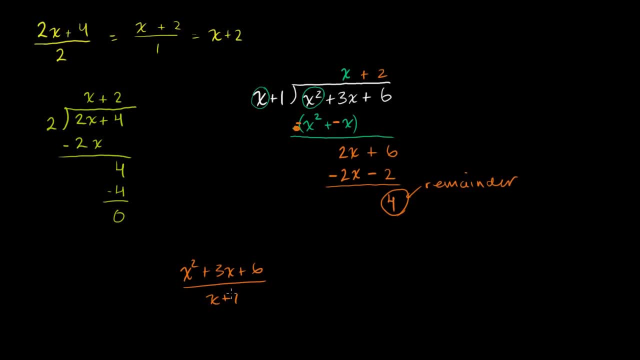 x plus 1.. Notice: this is the same thing as x squared plus 3x plus 6 divided by x plus 1.. This thing divided by this, We can now say that this is equal to x plus 2.. It is equal to x plus 2 plus the remainder divided by x plus 1.. 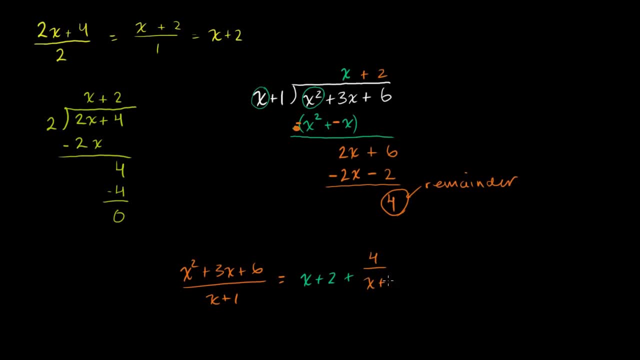 Plus 4 over x plus 1.. This right here and this right here are equivalent And if you want To check that, If you wanted to go from this back to that, what you could do is multiply this by. You could multiply it by x plus 1 over x plus 1.. 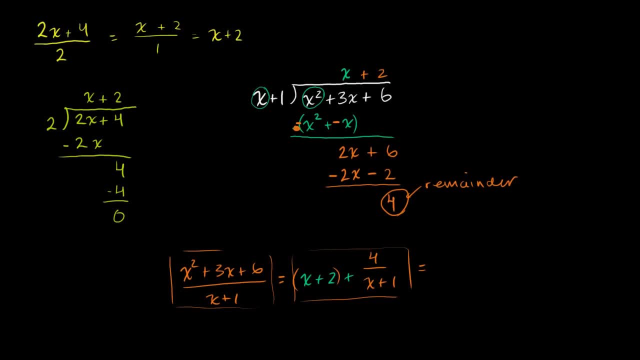 And then add the two. So this is the same thing as x plus 2.. And I'm just going to multiply that times x plus 1 over x plus 1, right, That's just multiplying it by 1.. And then to that add 4 over x plus 1.. 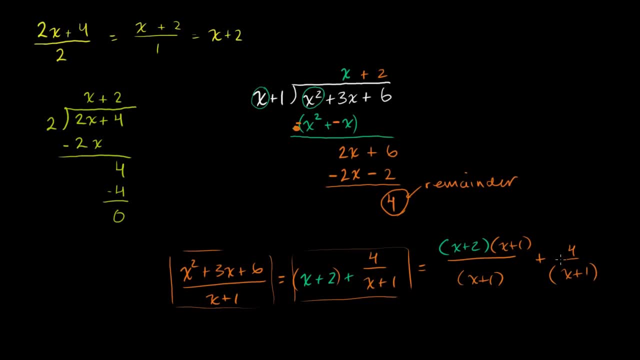 I did that, So I have the same common denominator. And when you perform this addition right here, when you multiply these two binomials and then add the 4 up here, you should get x squared plus 3x plus 6.. 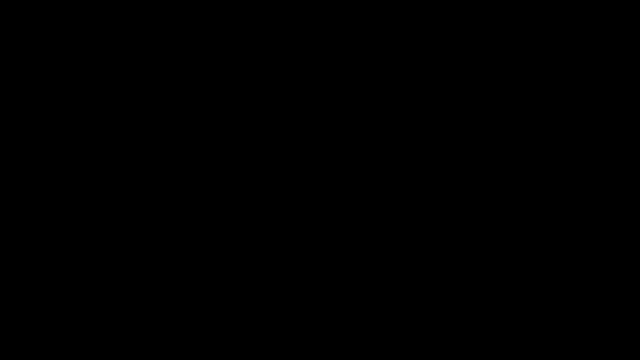 Let's do another one of these. They're kind of fun. So let's say that we have. We want to simplify x squared plus 5x plus 4 over x plus 1.. So once again we can do our algebraic long division. 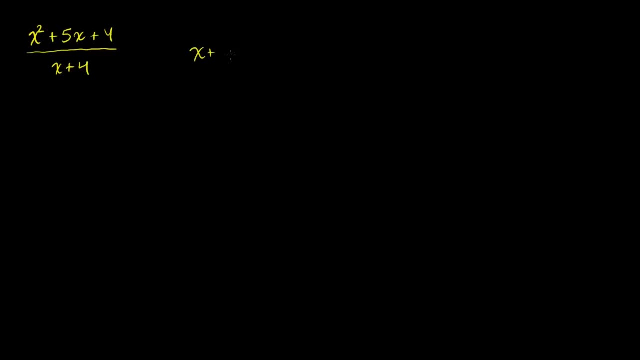 We can divide x plus 4 into x squared plus 5x plus 4.. And once again, same exact process. Look at the highest degree terms. In both of them, x goes into x squared. how many times It goes into it? x times. 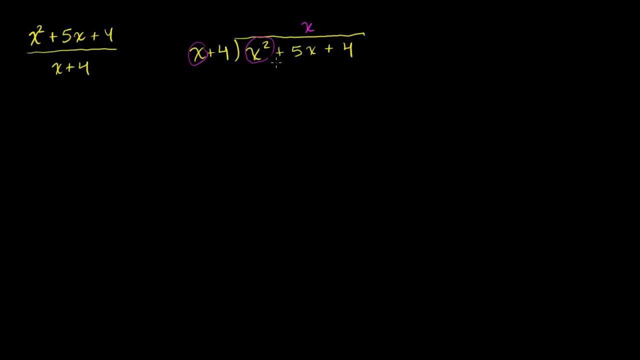 Put it in the x place. This is our x place right here. x times x is x. squared, x times 4 is 4x, And then, of course, we're going to want to subtract these from there, So let me just put a negative sign there. 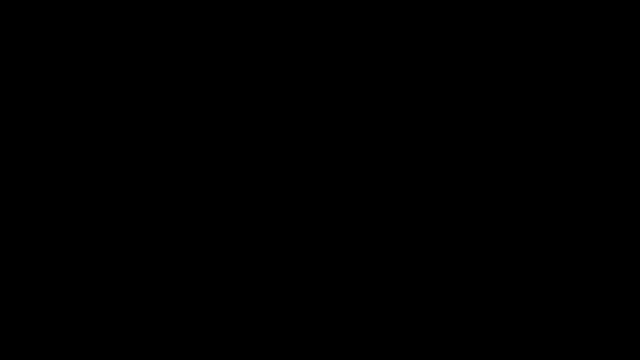 So let's say that we have. we want to simplify x squared plus 5x Plus 4 over x plus 4.. So once again we can do our algebraic long division. We can divide x plus 4 into x squared plus 5x plus 4.. 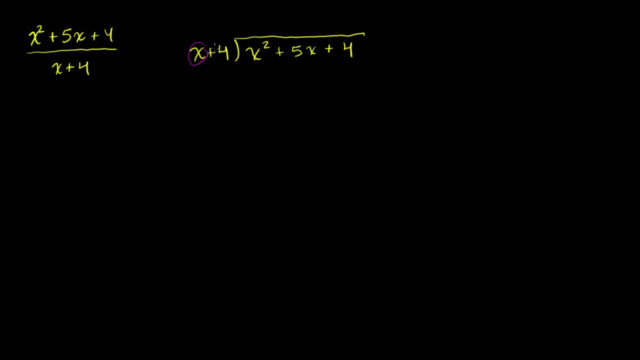 And once again, same exact process. Look at the highest degree terms. in both of them, x goes into x squared. How many times It goes into it? x times Put in the x place. This is our x place right here: x times x is x squared. 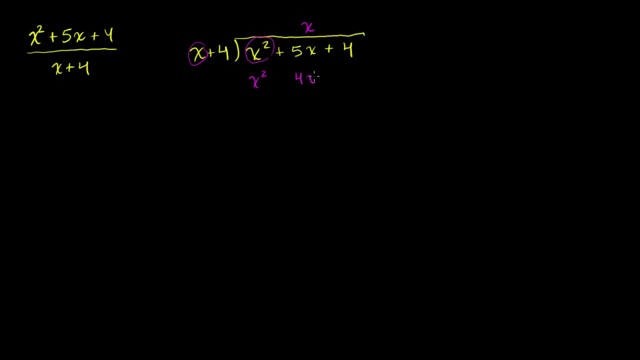 x times 4 is 4x, And then of course we're going to want to subtract these from there. So let me just put a negative sign there, And then these cancel out: 5x minus 4x is x. 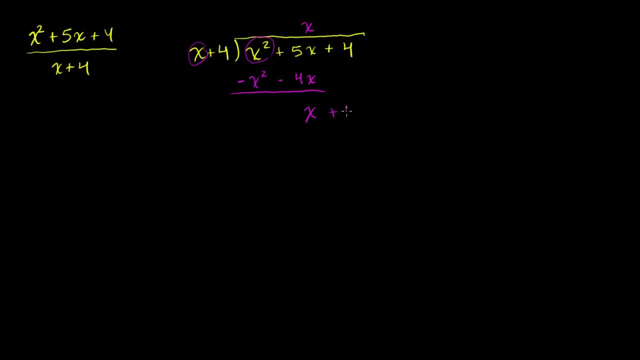 4 minus 0 is plus 4.. x plus 4, and you could even see this coming. You could, Let's say: x plus 4 goes into x plus 4,, obviously one time. Or you could just look at, if you were not looking at, the 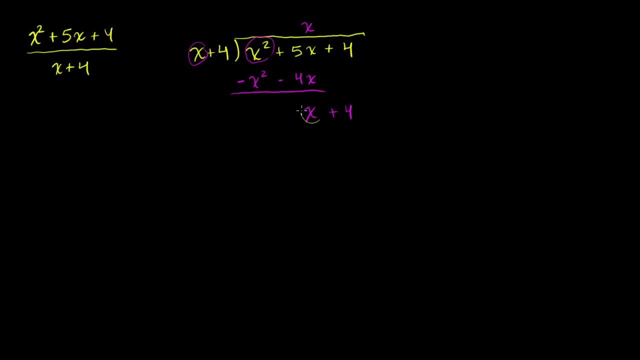 constant terms, you would completely just say: well, x goes into x. how many times? Well, one time Plus 1.. 1 times x is x, 1 times 4 is 4.. We're going to subtract them from up here. 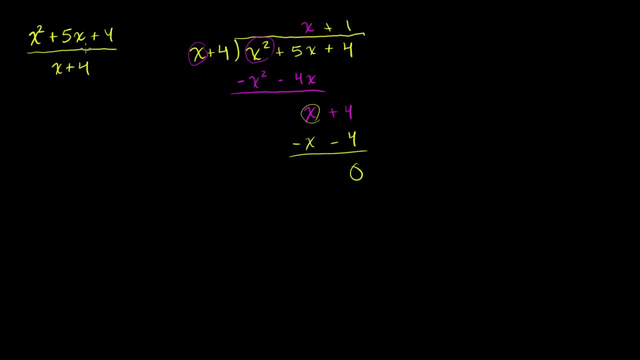 So it cancels out, So we have no remainder. So this right here simplifies to this: is equal to x plus 1.. And there's other ways you could have done this. We could have tried to factored this numerator x squared plus 5x plus 4, over x plus 4.. 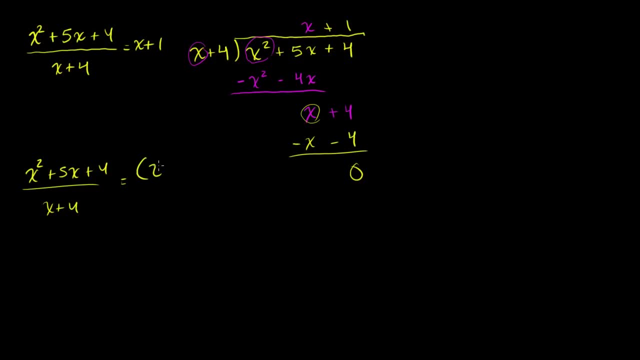 This is the same thing as what We could have factored this numerator as: x plus 4 times x plus 1.. 4 times 1 is 4.. 4 plus 1 is 5.. All of that over x plus 4.. 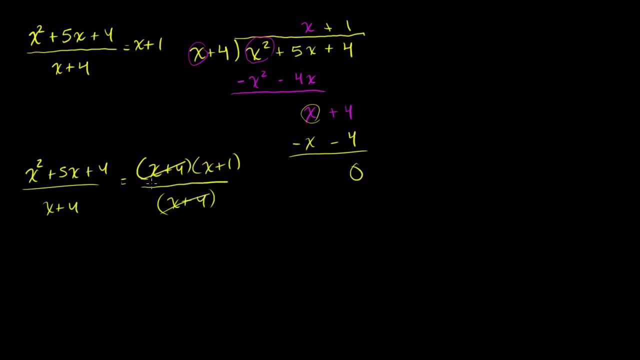 That cancels out and you're left just with x plus 1.. Either way would have worked, but the algebraic long division will always work, Even if it's not a perfect. if you can't cancel out factors like that, even if you did have a remainder in this situation. 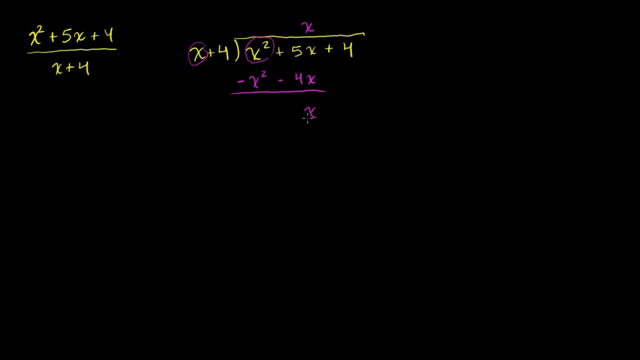 And then these cancel out: 5x minus 4x is x, 4 minus 0 is plus 4.. x plus 4, and you could even see this coming: You could say: x plus 4 goes into x plus 4, obviously one. 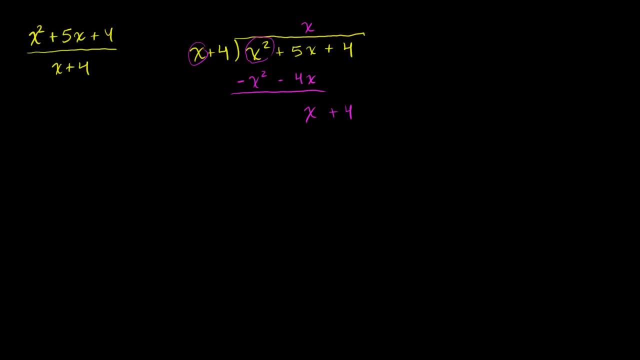 time, or you could just look at. if you were not looking at the constant terms, you would completely just say: well, x goes into x. how many times? Well, one time Plus 1.. 1 times x is x. 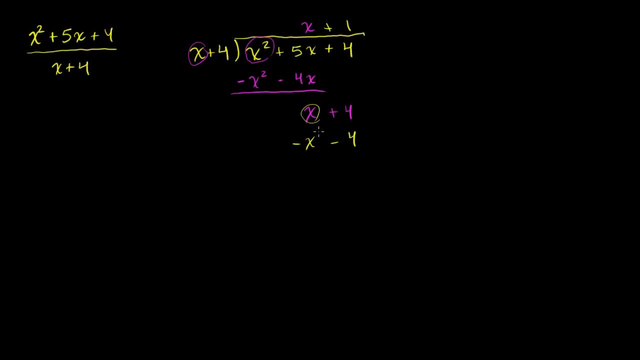 1 times 4 is 4.. We're going to subtract them from up here, So it cancels out, So we have no remainder. So this right here simplifies to this: is equal to x plus 1.. And there's other ways you could have done this. 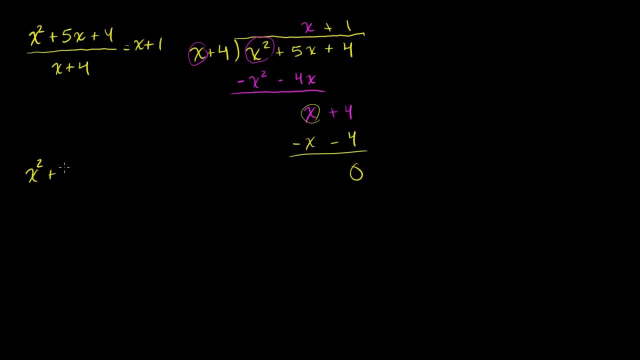 We could have tried to factor this numerator x squared plus 5x squared Plus 4, over x plus 4.. This is the same thing as what We could have factored this numerator as x plus 4 times x plus 1.. 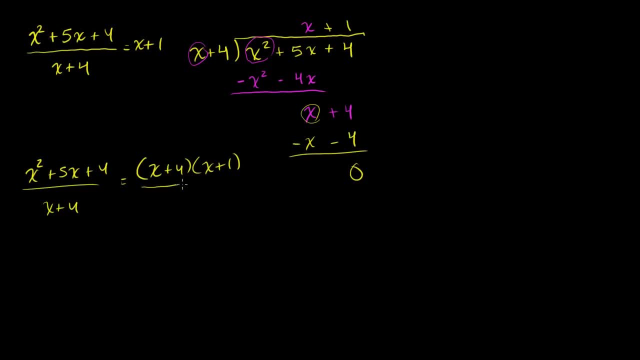 4 times 1 is 4.. 4 plus 1 is 5.. All of that over x plus 4.. That cancels out and you're left just with x plus 1.. Either way would have worked, but the algebraic long. 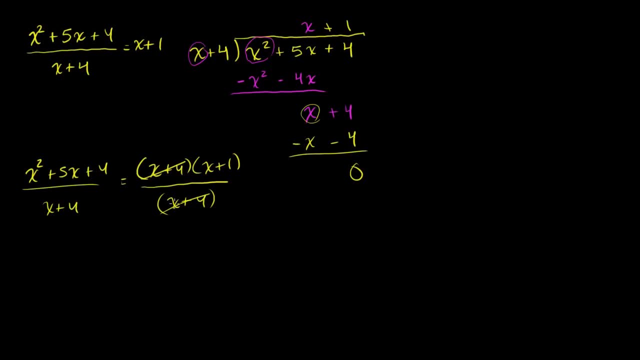 division will always work, even if it's not a perfect, if you can't cancel out factors like that. even if you did have a remainder In this situation, you didn't, So this was equal to x plus 1.. Let's do another one of these. 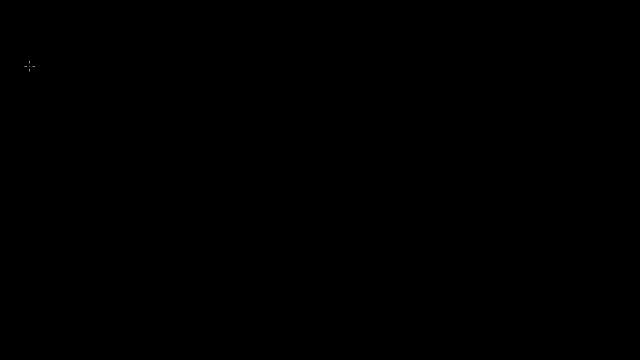 Because this is actually a very, very useful skill to have in your toolkit. So let's say we have x squared. Let me just change it up. Let's say we had 2x squared. I could really make these numbers up On the fly. 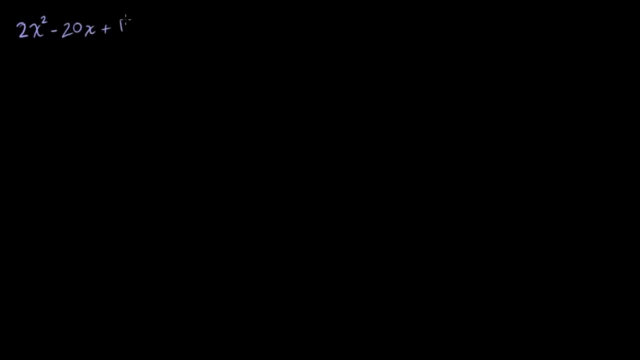 2x squared minus 20x plus 12 divided by actually. let's make it really interesting. Just to show you that it'll always work, I want to go above quadratic. So let's say we have 3x to the third minus 2x squared plus. 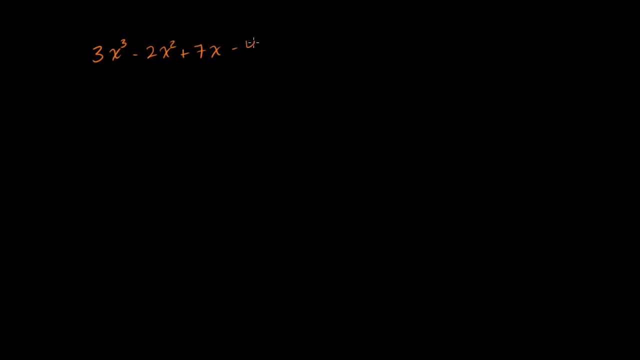 7x minus 4.. And we want to divide that by x squared plus 1.. OK, I just made this up, But we can just do the algebraic long division to figure out what this is going to be, Or what this is. if we simplify it, what it'll be. 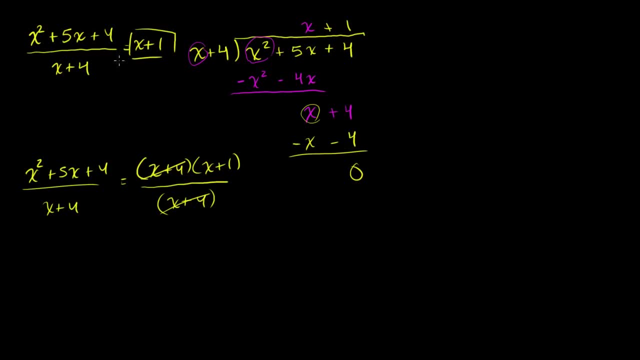 you didn't. So this was equal to x plus 1.. Let's do another one of these Just to make sure that you really have, because this is actually a very, very useful skill to have in your toolkit. So, let's say: we have x squared, we have, let me. let's say we. 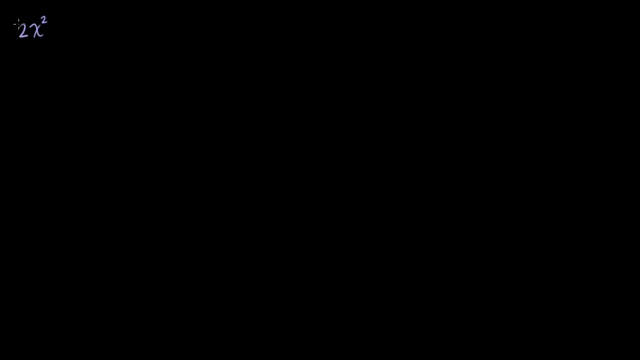 had. let me just change it up. Let's say we had 2x squared. I could really make these numbers up on the fly- 2x squared minus 20x, plus 12 divided by actually. let's make it really interesting. 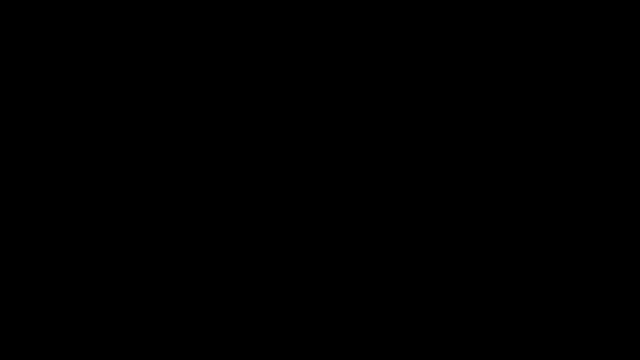 Just to show you that it will always work, I want to go above quadratic. So let's say we have 3x to the third minus 2x squared, plus 7x minus 4. And we want to divide that. We want to divide that. 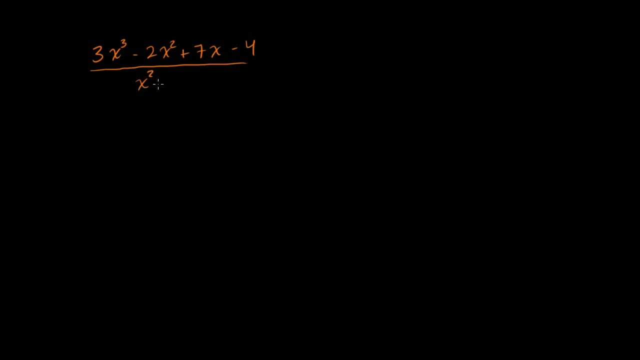 We want to divide that by x squared plus 1.. I just made this up. But we can just do the algebraic long division to figure out what this is going to be Or what this is. we simplify it what it'll be. 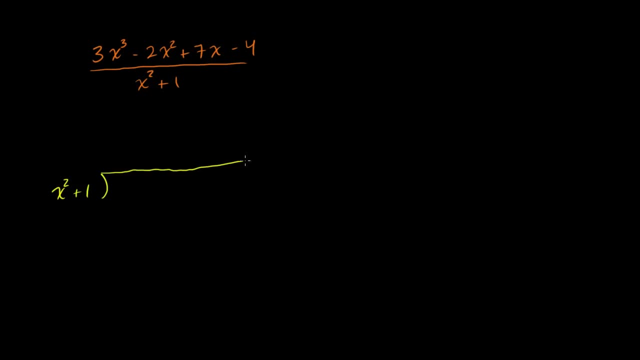 x squared plus 1, divided into this thing up here, 3x to the third, minus 2x squared plus 7x minus 4.. Once again, look at the highest degree term: x squared, It goes into 3x to the third. how many times 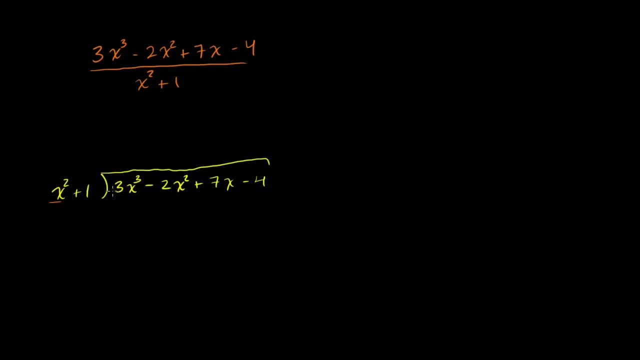 Well, it's going to go into it 3x times, right? You multiply 3x times this, you get 3x to the third. So it's going to go into it 3x times. So you have to write the 3x over here in the x term. 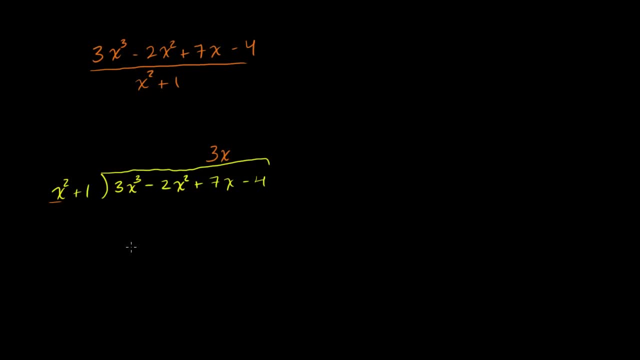 So it's going to go into it 3x times, just like that. Now let's multiply 3x times x squared is 3x to the third right, 3x times x squared Plus 3x times 1.. 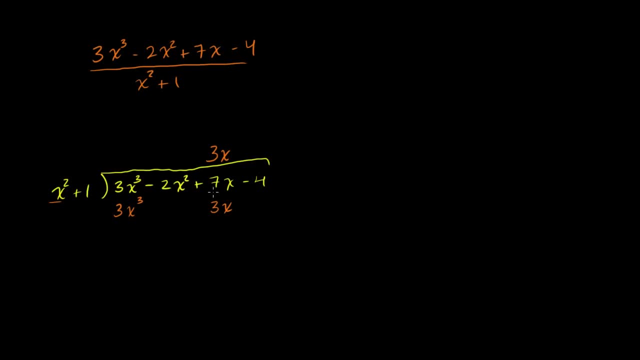 So we have a 3x over here- I'm making sure to put it in the x place- And we're going to want to subtract them. And what do we have? What do we have when we do that? These cancel out. 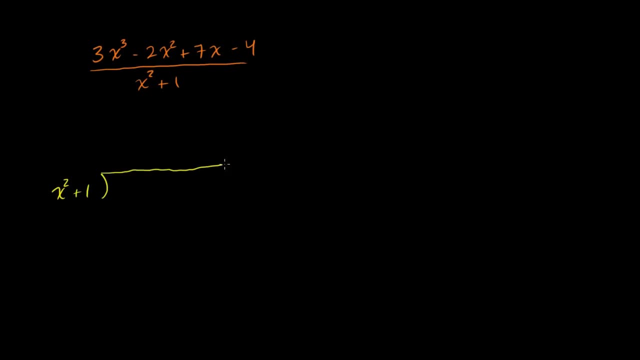 x squared plus 1, divided into this thing up here, 3x to the third, minus 2x squared plus 7x minus 4.. Once again, look at the highest degree term. x squared goes into 3x to the third. how many times 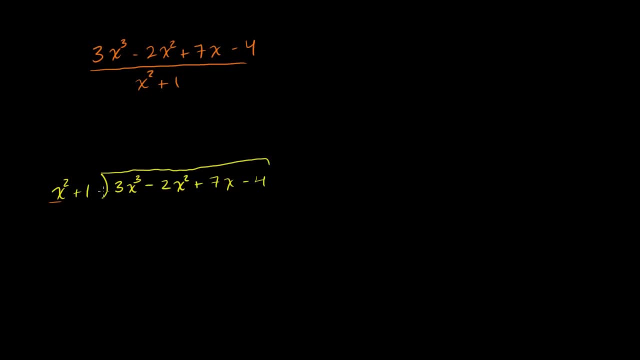 Well, it's going to go into it. 3x to the third, x times, right? You multiply 3x times this, you get 3x to the third. So it's going to go into it 3x times. 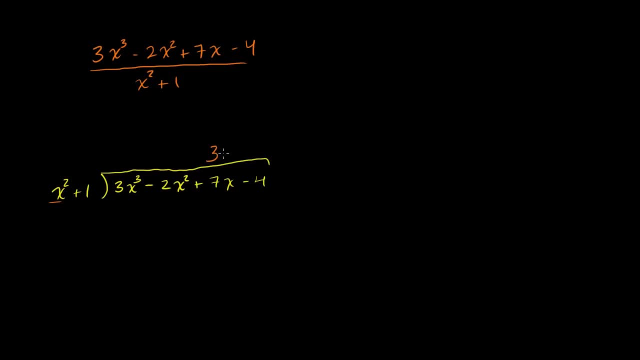 So you have to write the 3x over here in the x term, So it's going to go into it 3x times, just like that. Now let's multiply 3x times. x squared is 3x to the third right. 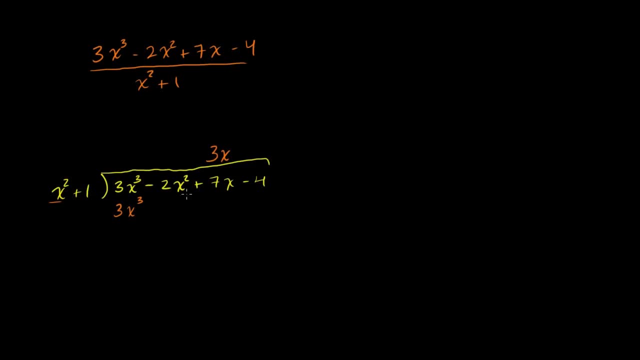 3x times x, squared plus 3x times 1.. So we have a 3x over here- I'm making sure to put it in the x place- And we're going to want to subtract them. And what do we have? 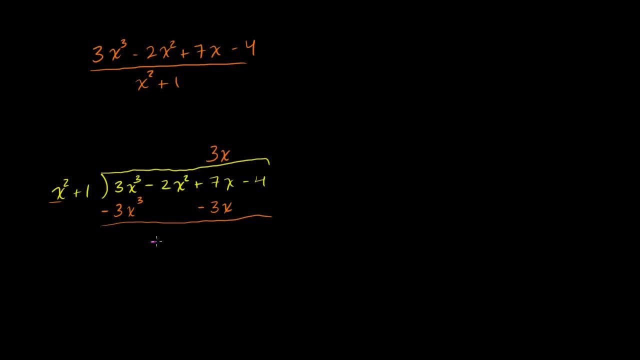 What do we have when we do that These cancel out? We have a minus 2x squared And then 7x minus because I just subtracted 0 from there. 7x minus 3x is plus 4x. 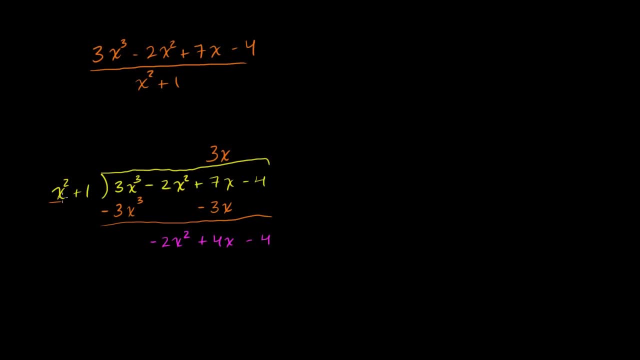 And we have a minus 4.. Once again, look at the highest degree term, x squared and a negative 2x squared. So x squared goes into negative, 2x squared, negative 2 times Negative. 2. Put it in the constant place. 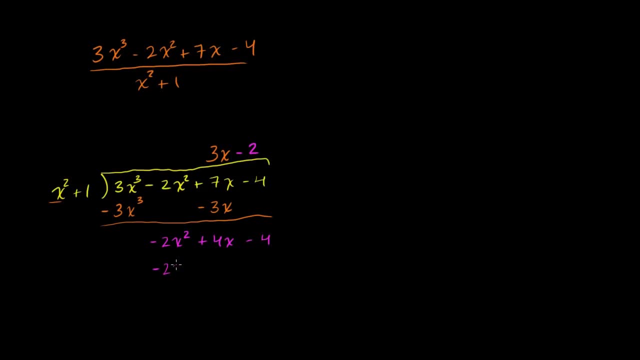 Negative 2 times x squared is negative 2x squared. Negative 2 times 1 is negative 2. Negative 2.. Now we're going to want to subtract these from there, So let's multiply them by negative 1,. 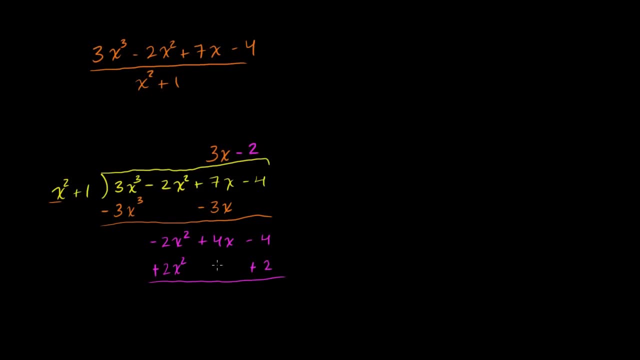 or those become a positive. These two guys cancel out. 4x minus 0 is 4x minus. let me switch colors. 4x minus 0 is 4x. 4x minus 0 is 4x. 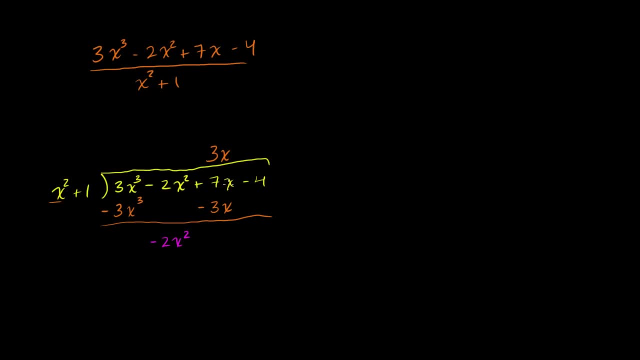 We have a minus 2x squared And then 7x minus, because I just subtracted 0 from there. 7x minus 3x is plus 4x And we have a minus 4.. Once again, look at the highest degree term. 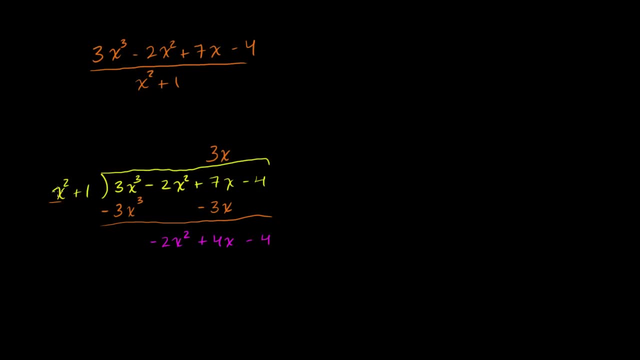 x squared And a negative 2x squared. So x squared goes into negative, 2x squared: negative 2 times Negative 2. Put it in the constant place: Negative 2 times x squared is negative 2x squared. Negative 2 times 1 is negative 2.. 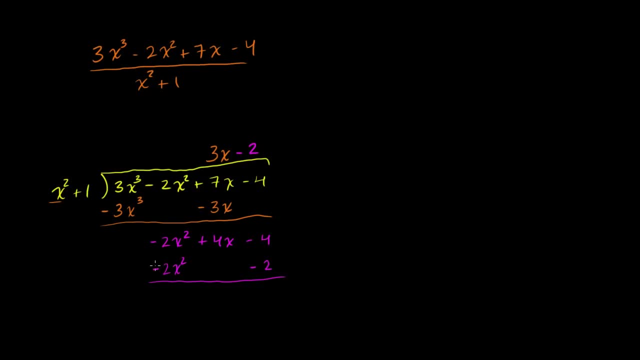 Now we're going to want to subtract these from there. So let's multiply them by negative 1, or those become a positive. These two guys cancel out 4x minus 0.. Is 4x minus? let me switch colors. 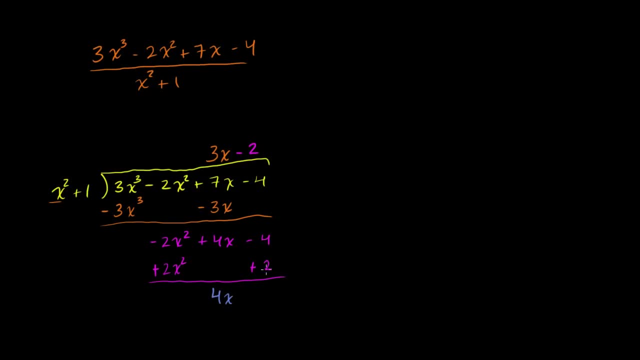 4x minus 0 is 4x. Negative. 4 minus negative 2, or negative 4 plus 2, is equal to negative 2.. And then x squared now has a higher degree than 4x and the highest degree here. 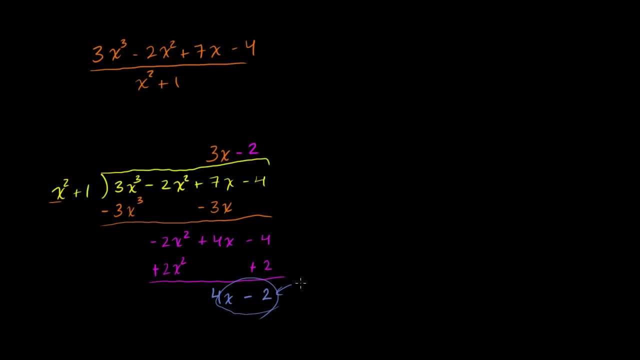 So we view this as the remainder. So this expression, we could rewrite it as being equal to 3x minus 2.. That's the 3x minus 2.. Plus our remainder, 4x minus 2.. All of that over x squared plus 1.. 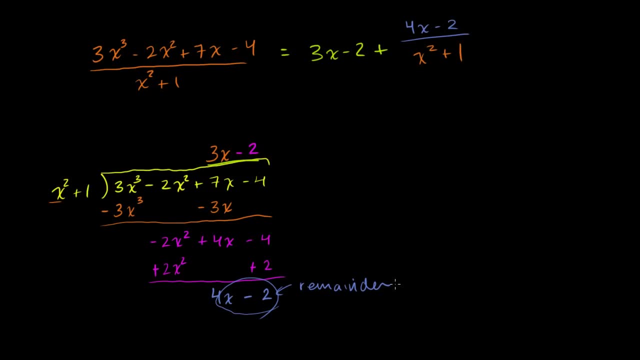 x squared plus 1. Hopefully you found that as fun as I did. 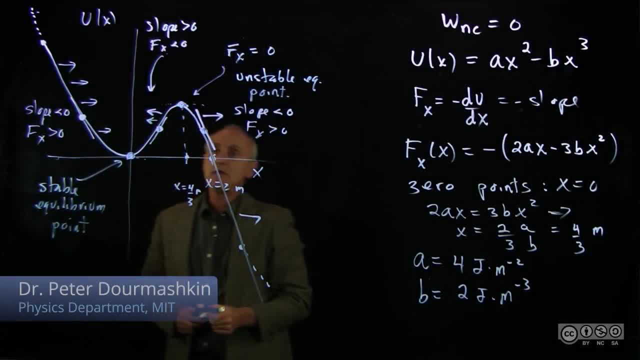 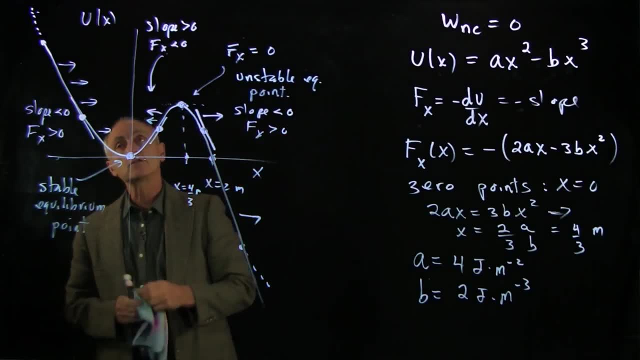 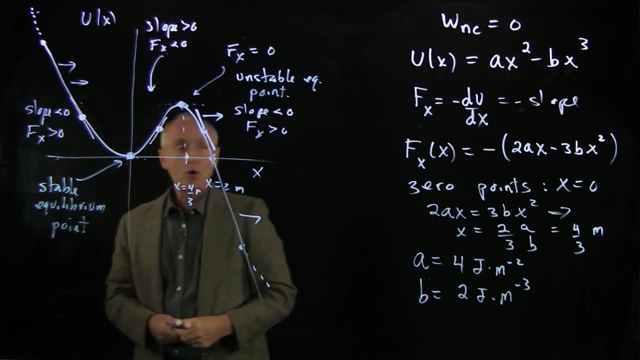 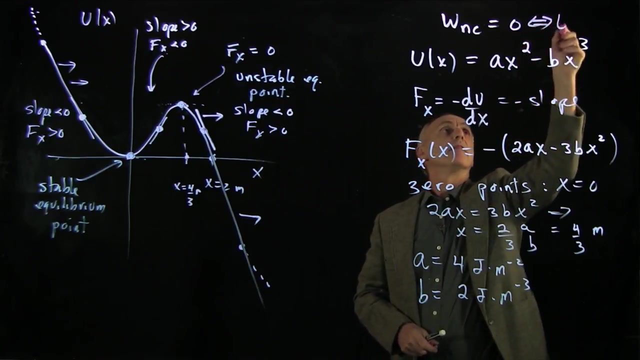 There's even a little bit more that we can learn about our energy diagram And I like to just clean this diagram up for a little bit of a second because I want to work in this area. Suppose our system, because the work non-conservative is zero, tells us that 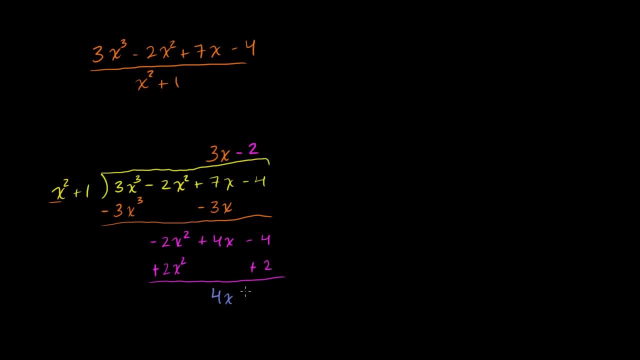 Negative 4 minus negative 2, or negative 4 plus 2, is equal to negative 2.. And then x squared now has a higher degree than 4x and the highest degree here. So we view this as the remainder.